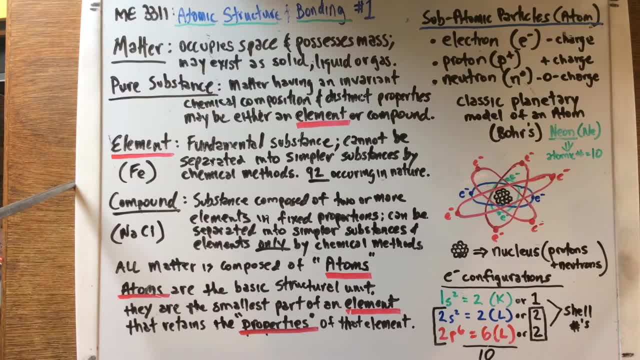 will be kind of a hybrid. It's going to be a hybrid mixture of some of these YouTube whiteboard lectures and, hopefully, some from the classroom, with a full board and a full time slot. So we'll do the best we can and we'll get through everything. So let's get started. 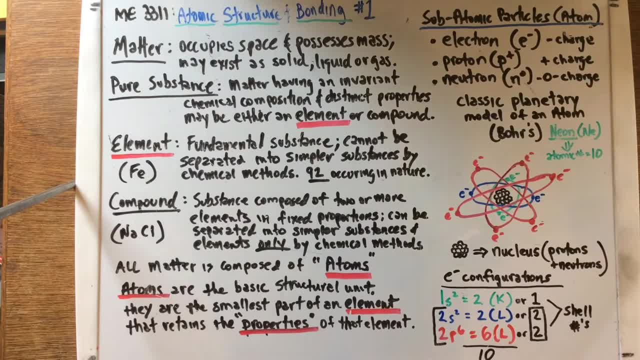 Okay, as I said, this is- and, by the way, my name is George Gray. I forgot to mention that on the first little introduction video and it's George Gray, G-R-A-Y, and here to your instructor and to help you get through this and to learn as much as you can with. 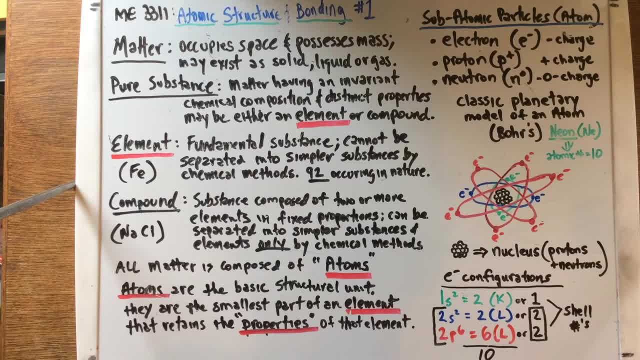 respect to materials and the methodology in selecting the correct material for the application. All right, so it all starts with matter of course. Matter generally occupies space, possesses mass, can exist either as a solid or liquid or a gas, and then it can be broken down into. 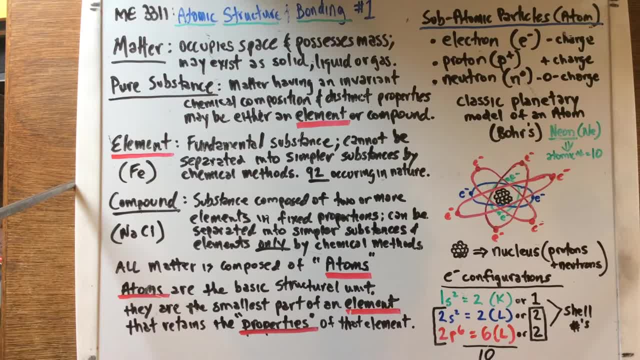 a pure substance or what we call a mixture. but we're going to go basically talking, emphasize pure substances and from that we can break that down into further two categories. So a pure substance is matter having an invariant chemical composition, which means it doesn't. 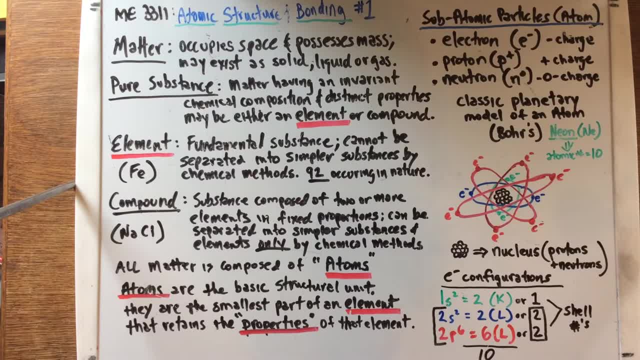 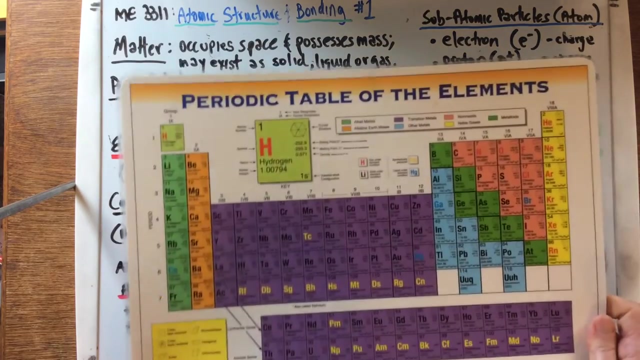 change and it has distinct properties. It can maybe be either an element or a compound, These pure substances. Now, an element is simply the fundamental substance that cannot be broken down or separated into any simpler substances by any chemical methods. and of course you recognize elements because they are cleverly on the periodic table of elements. 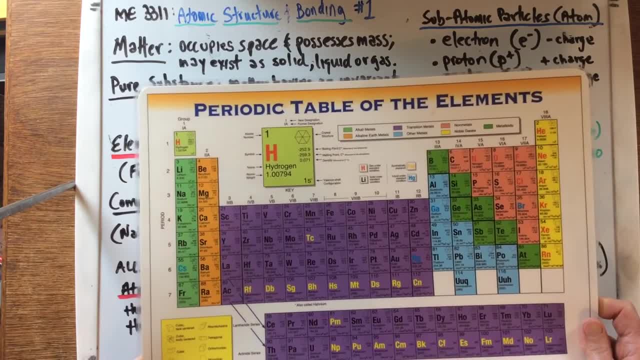 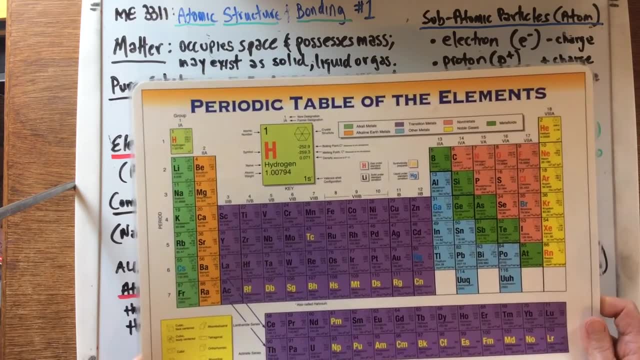 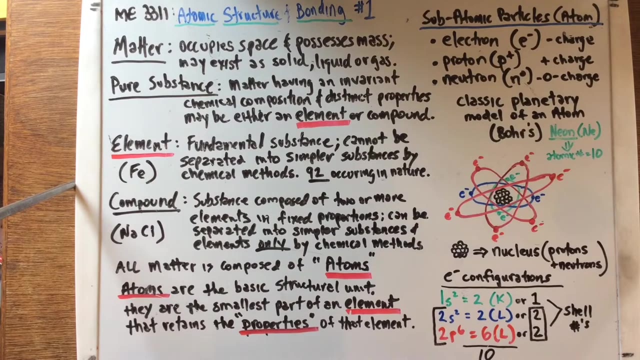 and we will go through that table in a short amount of time, Probably not today, but the next one. we will cover the periodic table of elements Now. I picked iron right here in the middle, here, of course, and iron is a pure element. 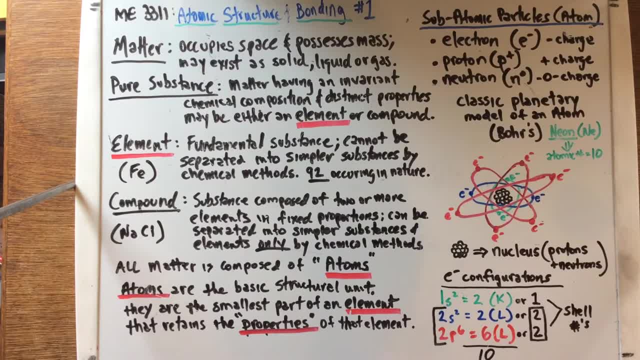 and of course there are about 92 occurring in nature, 92 elements occurring. There's many more, but those are kind of synthesized and not really occurring in nature, so we'll concentrate on the ones that are occurring in nature. Then there's compounds, so these 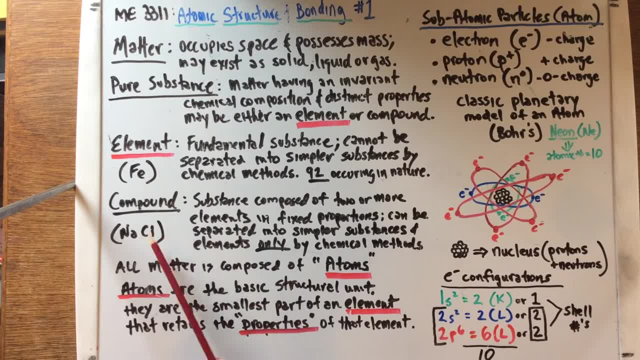 pure substances get broken down, So an element or a compound. a compound, basically, is a substance that's composed of two or more elements in very fixed proportions and can be separated into simpler substances and elements, but only by chemical methods, and a good example here would be sodium chloride or your local. 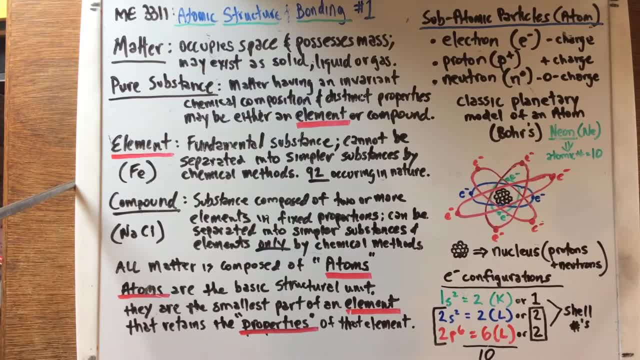 table salt. So of course, all matter is composed of atoms, all matter composed of atoms, and atoms are the basic structural units. And you know, I'm not going to go into too much detail on that, I'm just going to go. 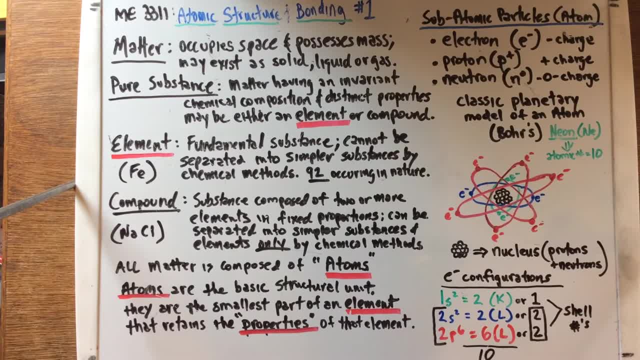 through it When building things, when building materials, et cetera. there's nothing smaller. It's the basic building block. It doesn't get any smaller than that. You can't split it in half or anything, of course, And so they're the smallest part of an element, and that smallest part retains the properties. 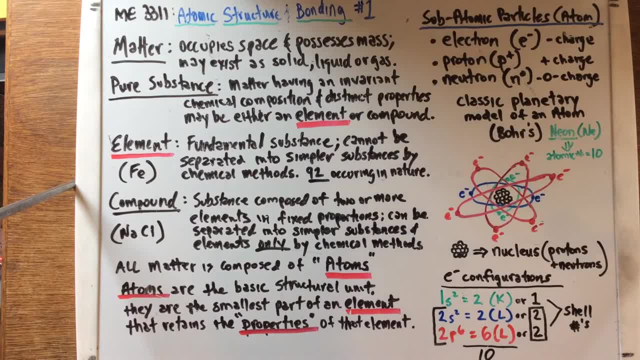 of that element, so it doesn't get any smaller than that. So I'm going to make sure you get a- I'll email you a handout on what I'm calling the atomic structure fundamentals And I'm going to cover a little bit of that right now and then I'll go over in detail. 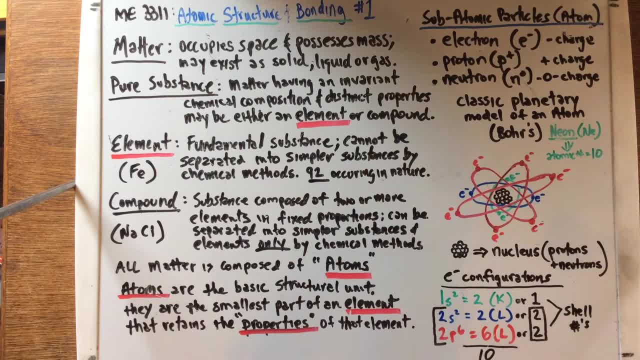 that handout a little bit later and I'll have that up on the board, that one way or the other. But let's talk about some subatomic particles And I'm not telling you anything you don't know already, just basically from your basic chemistry classes. but in an atom, of course, 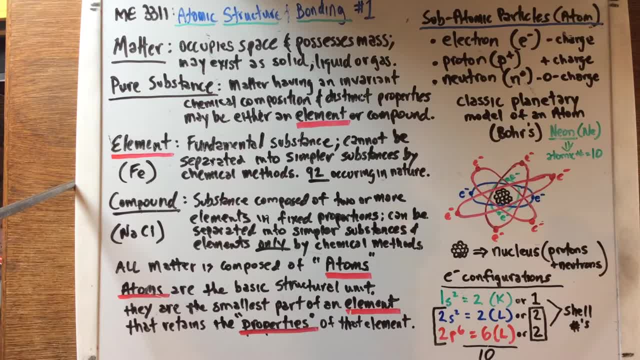 there are three subatomic particles, basically the electron, which is where everything happens, and of course the atom. So it's basically all of that, And then you have the atomic structure, and then you have, you know, the atomic structure, and then you have the subatomic particles. So basically, 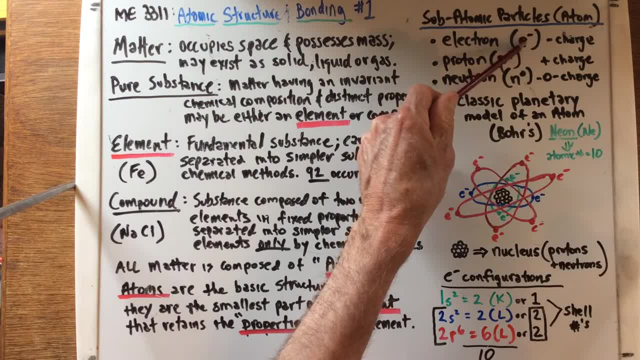 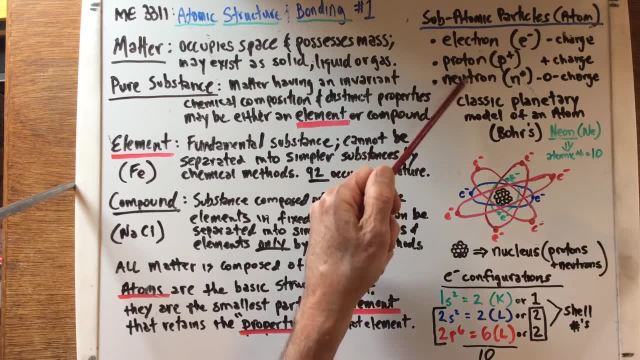 you don't know anything about it, but you understand that later. But let's talk about the subatomic particles. And of course it is a negative charge And here is the electron symbol, here And then within the nucleus, we have the proton and the neutron. 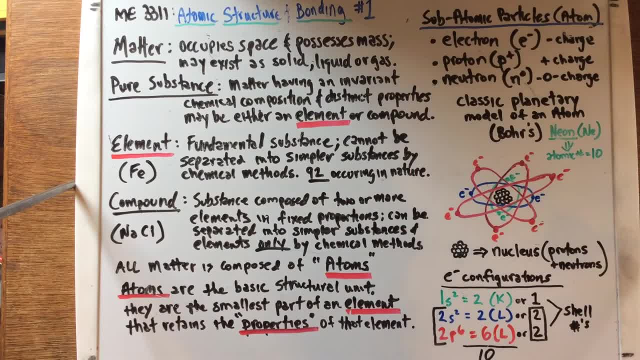 Of course, proton is positive charge, Neutron is zero charge, no charge, And so let's look at the structure of that, And we're looking at this as a basic structure that is following Bohr's planetary model of an atom, And the one we chose was neon. neon, right here. 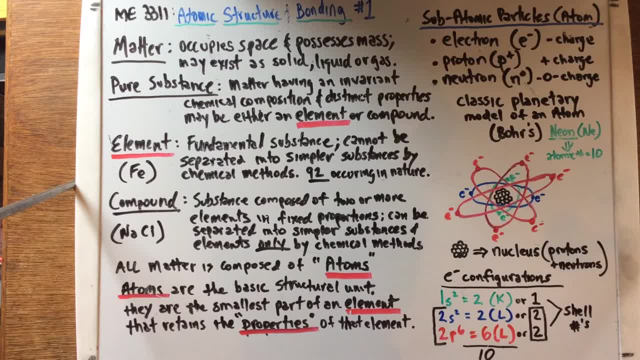 And it has an atomic number of 10, or also known as the proton number. But more about that later. Okay, so this is a representation. This is a representation of that again planetary model, what we know as Bohr's model of an atom. 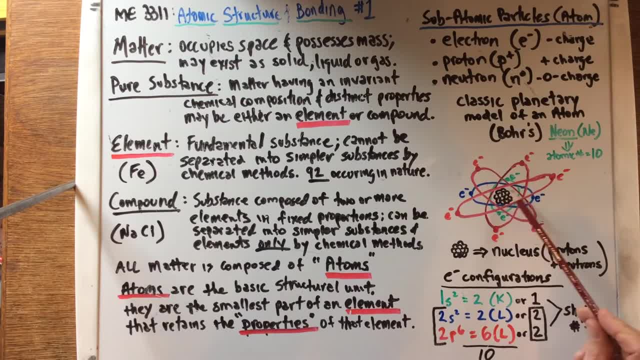 And this represents all these tiny little circles, represents the nucleus which, of course, is going to be comprised of the protons and neutrons in here All right now, as I said, where all the action is happening and where all the bonding takes place is with the electrons. 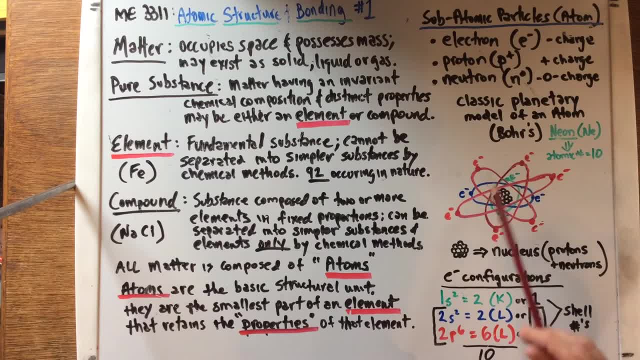 And these are these outer shells. They go around this nucleus And neon. since it has an atomic number of 10, it will have 10 electrons total in these shells. Now, these shells are very distinct. They all have distinct energy levels in these shells. 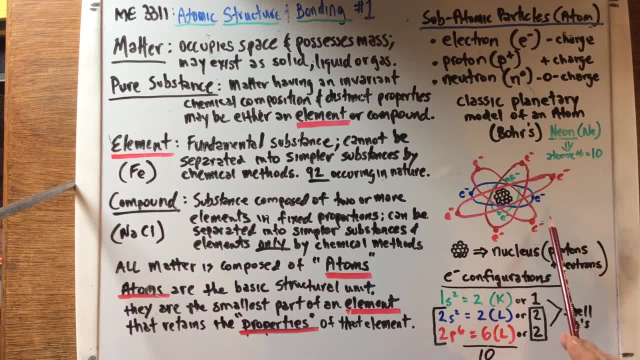 Each orbital has a very discrete energy level And they all kind of have a tendency to be the smallest or least Least energy first and then build up, And they're comprised in these different shells, or quantum shells like K, L and M, or shell 1,, 2, and 3,. 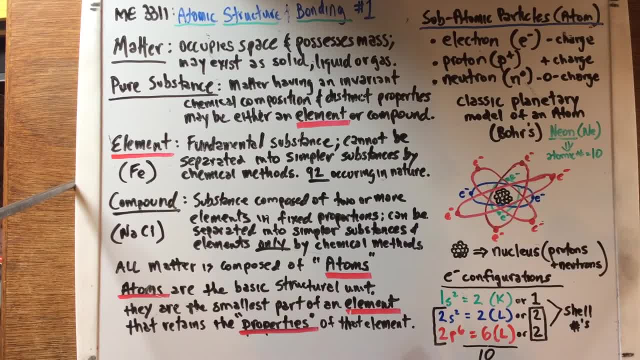 which is what I've got designated down here, But essentially what we're looking at here. the most important part of this, really, in dealing with bonding, is what the electron configurations look like, The disbursement of those electrons, The disbursement of those electrons throughout these different shells. 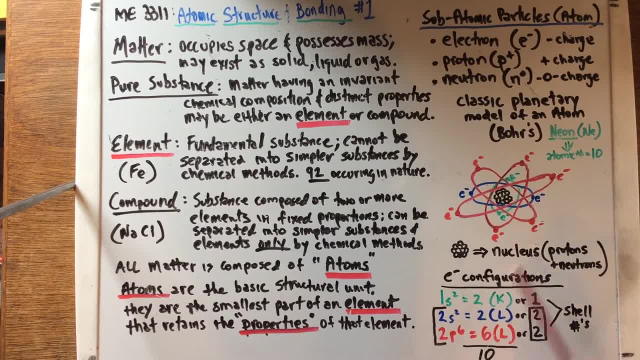 So if we look at neon- and I tried to color-code this, but the first shell is the S-shell- Now all of these shells have one orbital And each. the maximum number of electrons per orbital is 2.. That's the maximum. 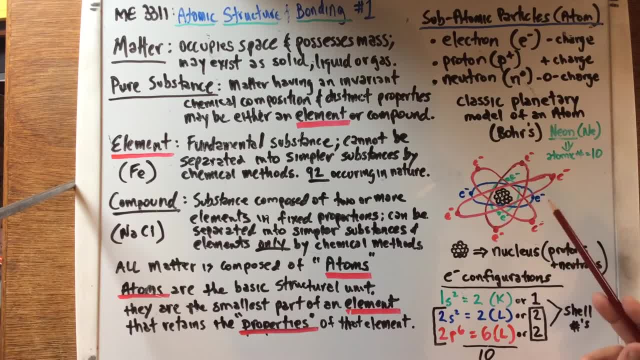 So what they do is they build up all these different shell numbers to build this up to a great number. So this first green little orbital, this first green little orbital, This first green little orbital around this nucleus, is the S-shell or S-orbital. 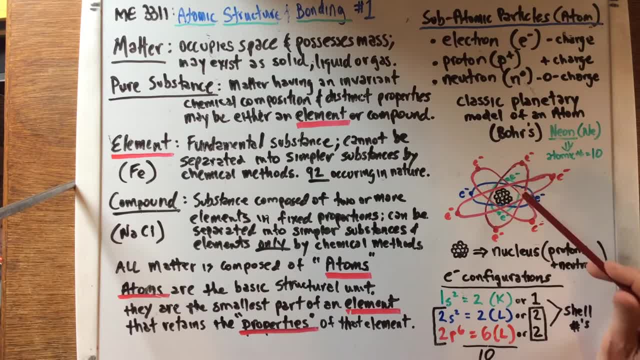 It has two potential electrons, and so it's obviously filled up because we need to get to a count of 10.. So this green shell is that first, and it's the S-shell. okay, And it's also known as the letter designation K. 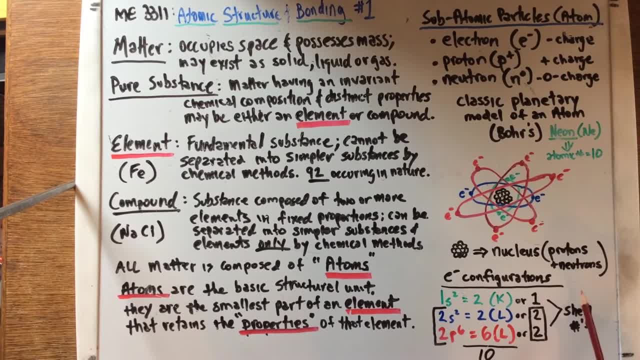 or what we're calling the first shell, or shell number 1.. Alright, so after that, that's all it can comprise. That first shell is just one. Now, the second shell has two orbitals. okay, It has an S-orbital and a P-orbital. 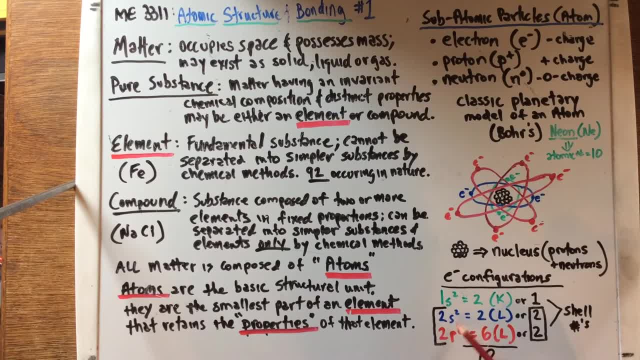 Well, the S-orbital only has two possible. The P-orbital has six possible because it has three of these orbitals here within this P-shell. So there's one, two, three, And so all three of these can contain. 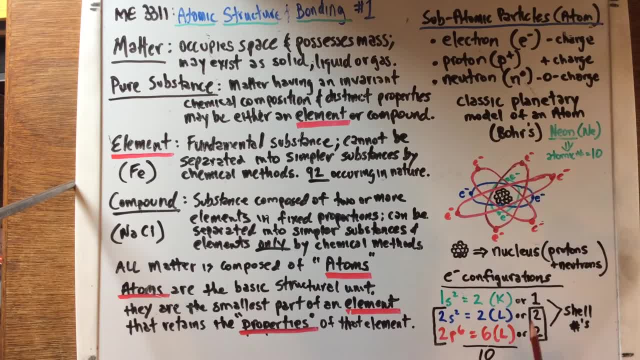 up to two electrons and they're completely full. So what we've got here, then, is the green first shell, S1S, and it's full, so it's 1S2, so that's the total of two electrons. 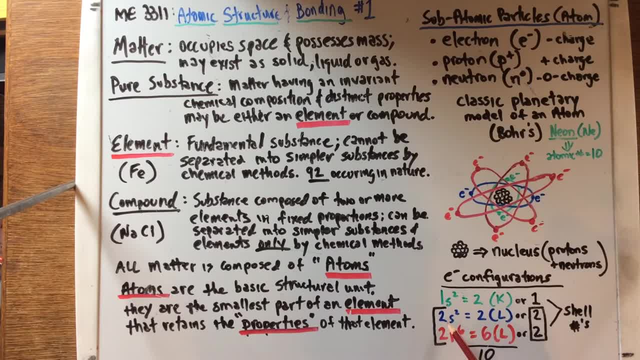 And then the second shell is just like this: 1S, but it's a 2S, and since it only can have two, that's again two. so that's two, four, and then the P. Now the P is still. 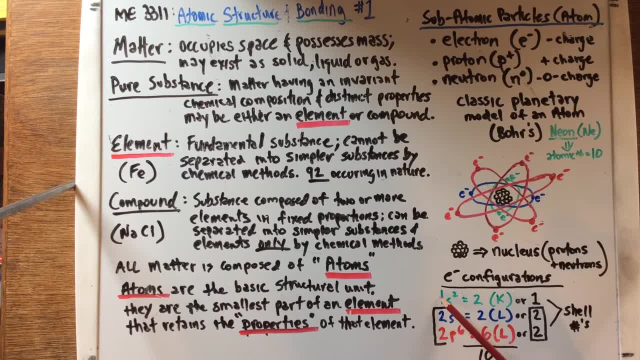 it's a two and it's designated as a 2S and a 2P, just like this is a 1S And we'll get into 3S, 3P etc. But the 2P has three of these orbitals. 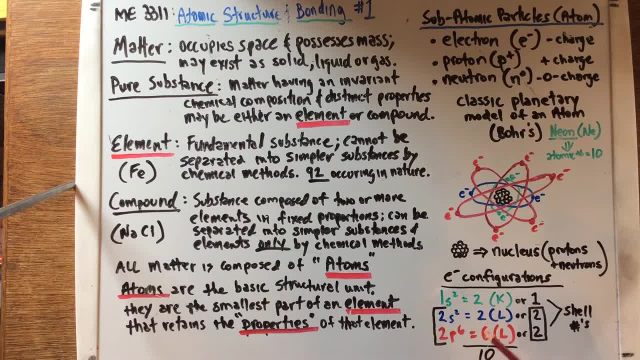 three of these shells here and again, they can only contain two each. So, and since this is 10, we're going to need six and of course, that's what we've got: Three orbitals, two each, that's six. 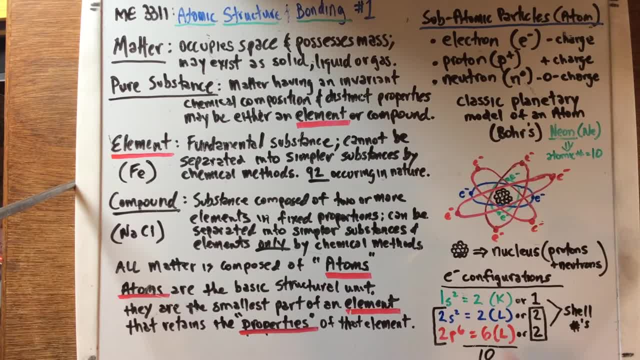 So we have two, four, six- that's 10, and 10 total. okay, So that is the completely stable or what we're calling an element in. that is a noble gas. since neon is a gas, It's what they call a noble gas or noble elements. 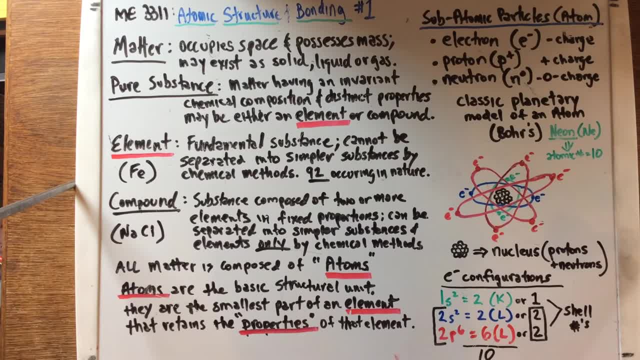 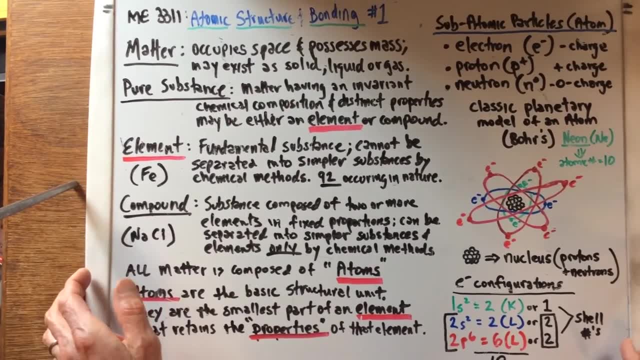 found in the far right-hand side of the periodic table of elements. So let's look at what these, let's look at some more examples of these electron configurations and we'll show you how these energy levels work. here, the energy states. 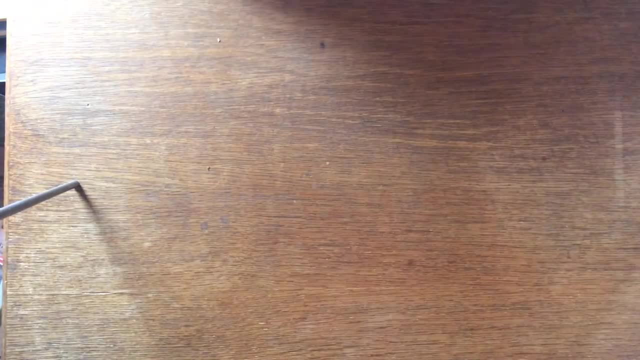 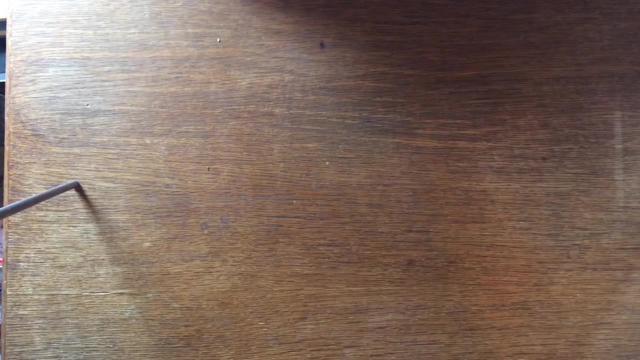 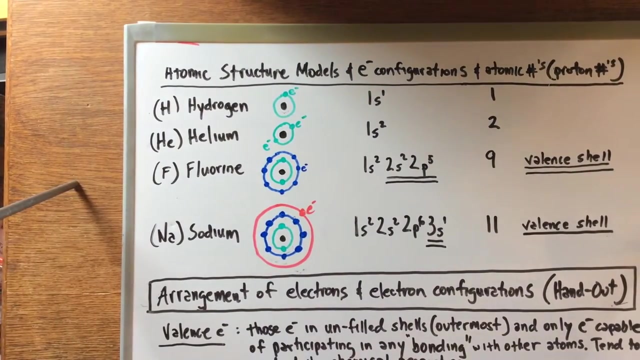 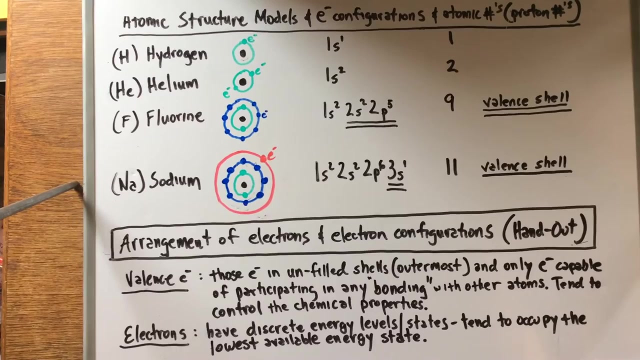 So let me remove this board And we'll put in another board. If I don't hit the frame, let me make sure it's all lined up here for you. Okay, I think that's pretty well. I think that's pretty good. 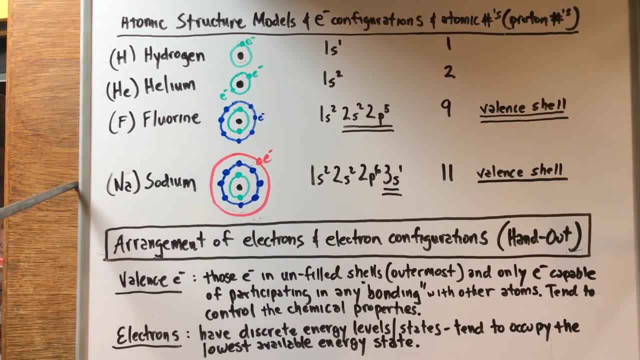 All right. So now let's look at some examples of some other elements and their electron configurations. So this is the models and the electron configurations and the atomic numbers. So start with, of course, the smallest, lightest, hydrogen. 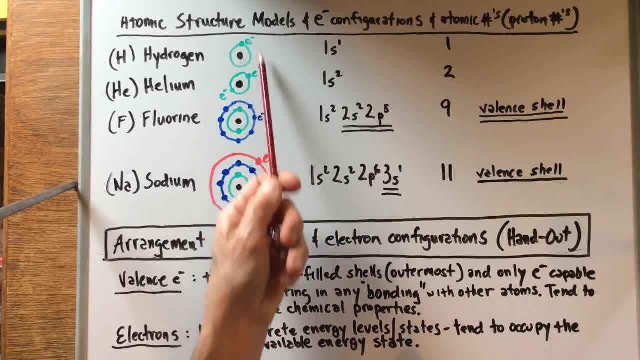 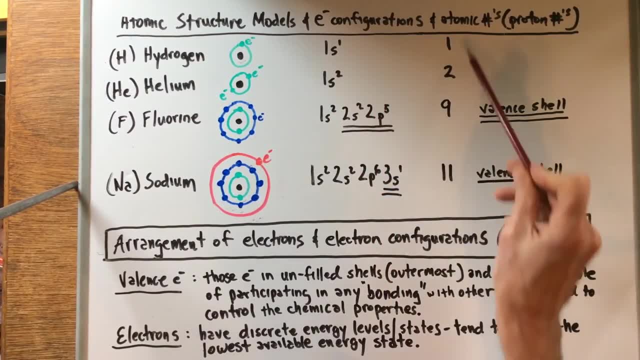 It has atomic number of one. So again, this 1s shell will just have one electron in it. So it's the electron designation would just be 1s1, and atomic number would be one. Okay, So helium moving all the way over again to that far side. 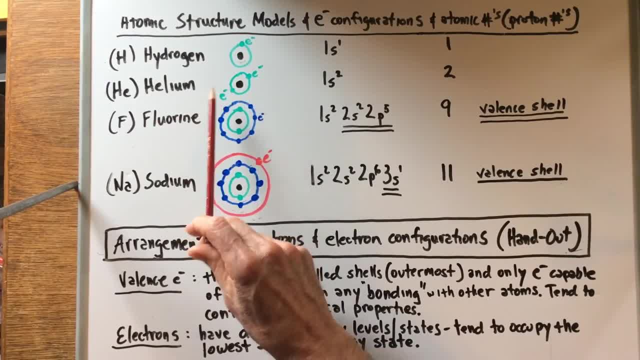 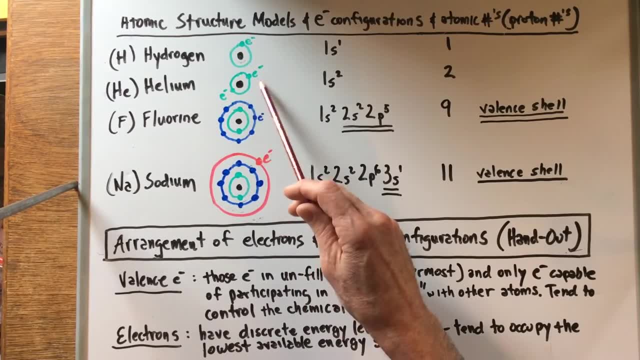 it's the next in order, So it has two and that 1s2.. So it's full. So helium is one of those noble gases because it cannot bond with anything, It has nothing to give, nothing to take. 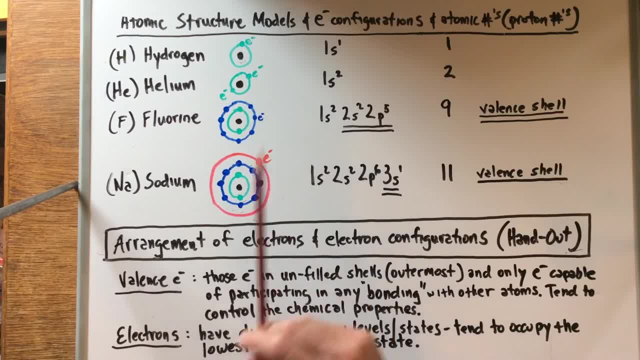 as far as the electrons, That's what most of the bonding is about, which we'll get into later- And so this has an atomic number. Helium has an atomic number of two. So let's move up a little bit. 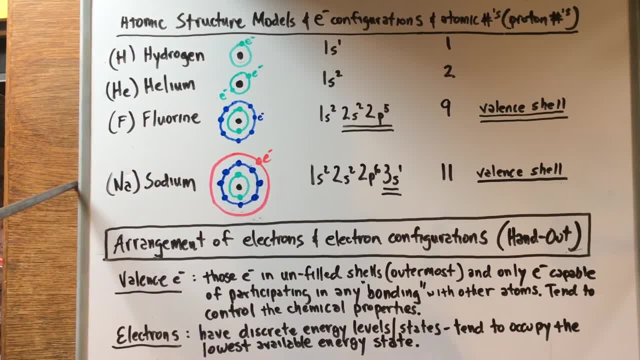 and let's go to an element known as fluorine. All right, Now again, it has an atomic number of nine, So we know we're going to have to get it above the 1s shell and the 2s shell. 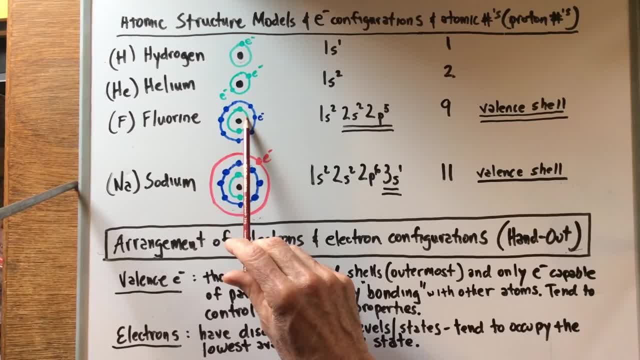 So let's look at this: The green again is that 1s shell, And then here is the two, which again has a potential of actually eight, because we have 2s2, and then this could be six. 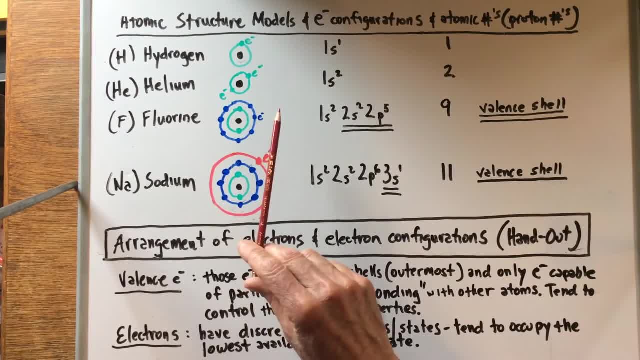 So it could be eight total. So here we have- actually we've got seven here, So we have 2s2, and what I'm not doing? I'm not showing the individual, like I did on the other screen. 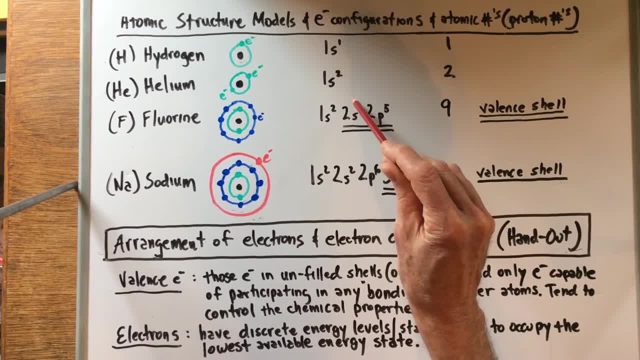 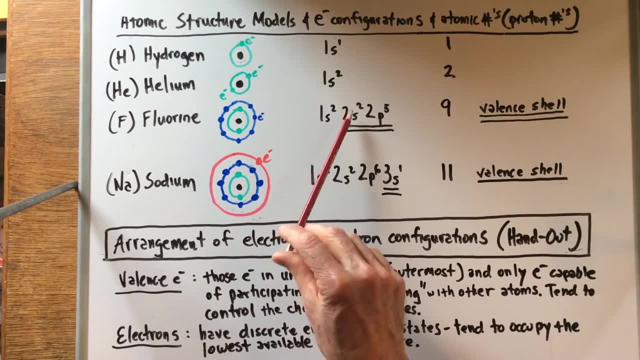 I'm just showing this as the 2s, which again potential of 2s2, 2p6, here. So this only needs, since the 2s2 would be full, of course, we'd only need five to get nine. 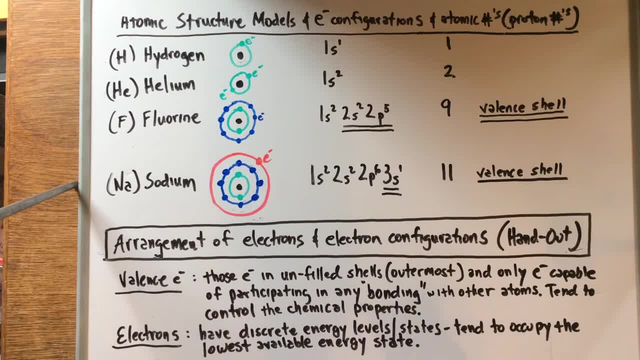 So there's one available, one available electron. So this is a very, very electron, has a very high electronegativity, I mean it is. it is needing only one more electron to complete its outer shell and become very stable. 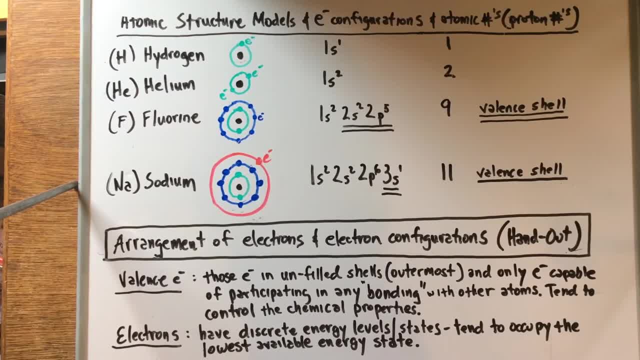 because that's ultimately what most elements are trying to do: is to become stable and have that outermost shell Completely full. So they're going to give away electrons if they don't have very many, or they're going to try to take. 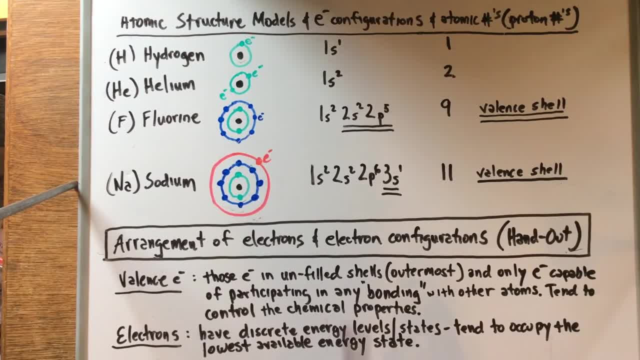 if they just need, you know just one. So, and that that talks more about the type of bonding that's involved, bonding that's involved which we'll get to. Alright, so its overall electron configuration would be 1s2, 2s2, 2p5.. 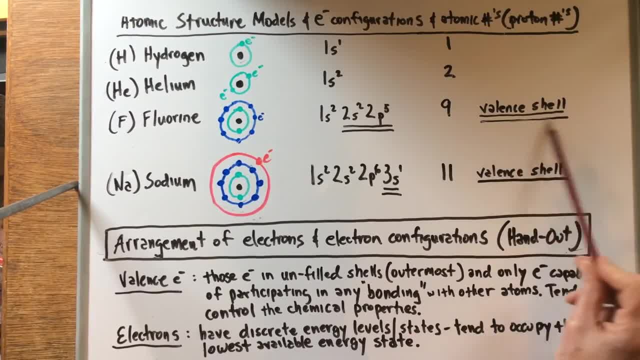 Alright, so it gives us a nine, And so this the the valence shell. here is this: This is the valence shell, This is the outer, outer shell, And this is the only shell that has any. 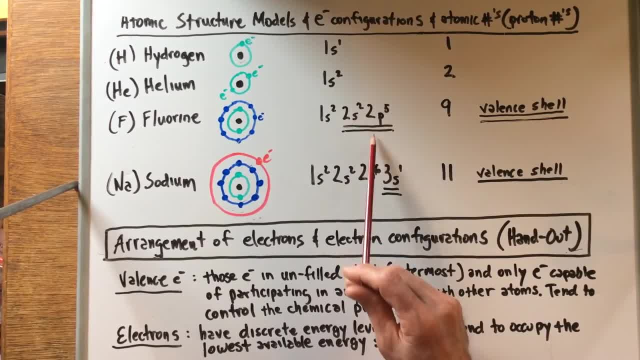 has any potential for doing any, any bonding or giving or taking away of electrons. It's always the outer shell. is referred to as the valence shell. Regardless of its, of its electron count, It's always the outermost shell, The complete shell. 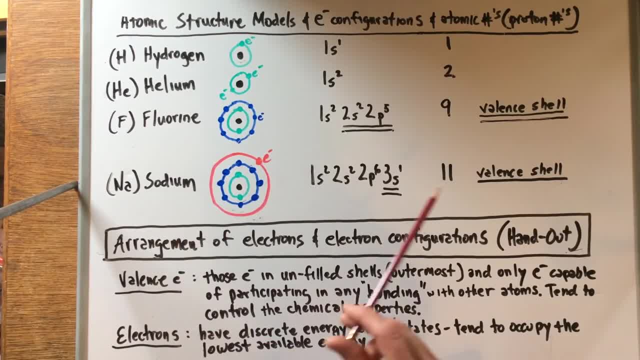 So let's move way up to sodium. here Sodium has an atomic number of 11.. So again we'll go through through the gyrations. here We've got 1s2, full, And then this 2s2 is completely full. 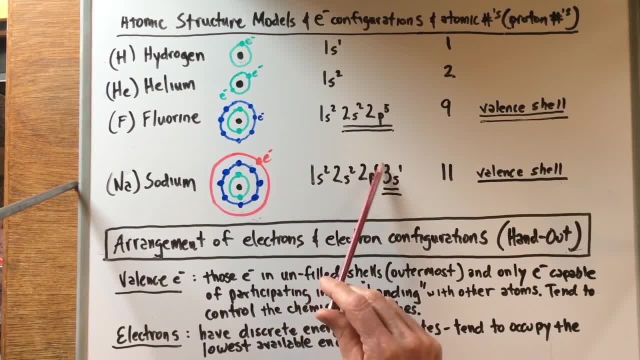 because we need 11.. So 2s2,, 2p6.. That's maxed out. The second shell is maxed out. So now we move into the third shell. The third shell, Which is M. The second shell is designated L. 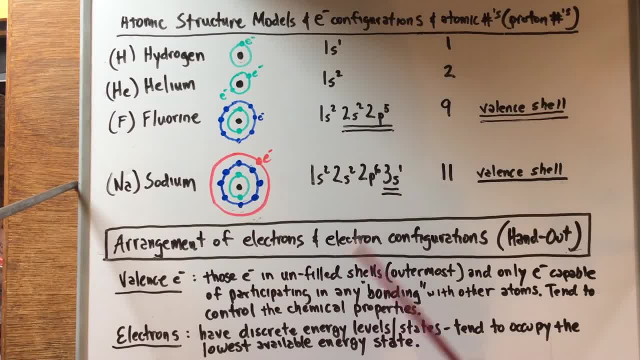 So we have K, L and M So far, And so we only need one electron. So we're only going to get to 3s1.. So again, it needs one more To satisfy this, To get this this out. 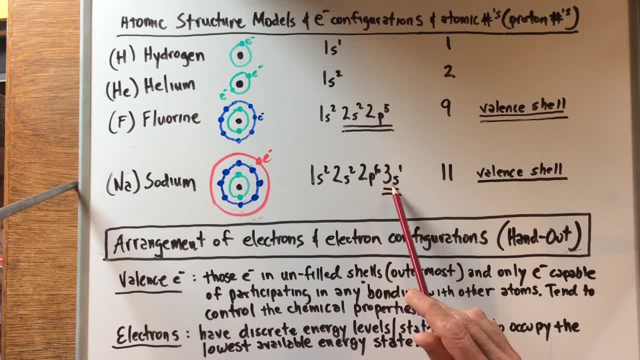 valence shell stable, And so, ultimately, the valence shell on this sodium is just the 3s1.. Alright, And that is the valence shell. That's the only one it can have to do any potential bonding with. So again, this is very important. 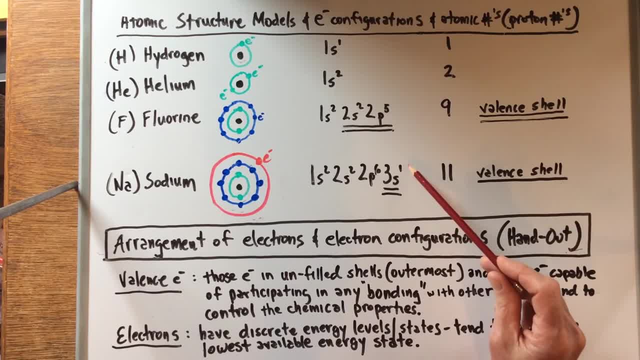 because the fact that this just has one needs one more. It's liable to give up one or take one, Depending on what's what's available, What's what's next, What it's trying to bond with And how it's going to bond. 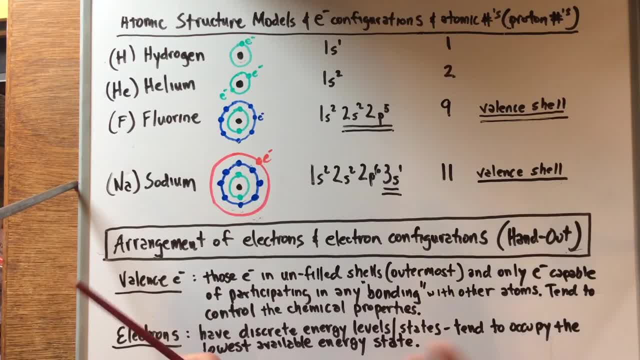 Whether, whether covalently sharing or ionic, Just transferring of those electrons. So I will go over this, Probably starting with this next lecture, Because I'm about to run out of time here, But I'll go over this arrangement of electrons. 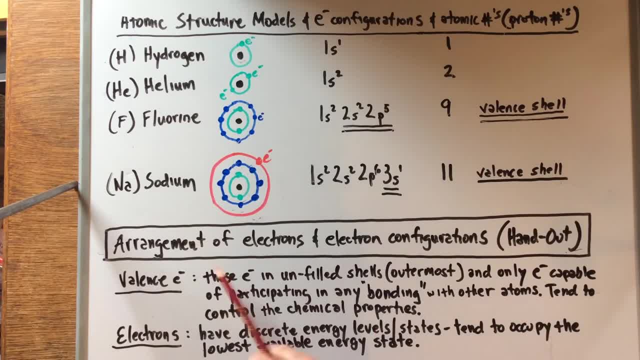 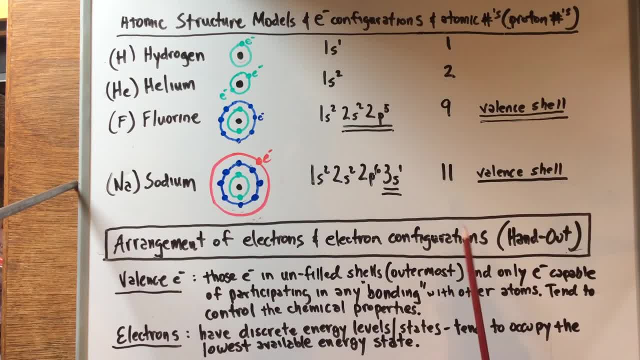 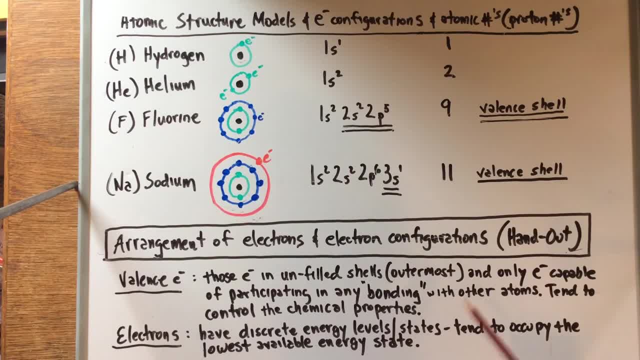 Those are the electrons in the unfilled shells, The outer most shells, And are the only editions capable of participating and doing any kind of bonding within the other atoms. And they tend, they also tend to control the chemical properties of those elements. So 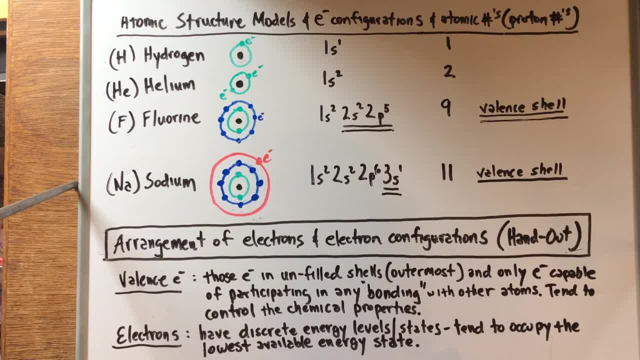 very, very important shells, known as the valence shells or valence electrons, And, as I told you before, these electrons have discrete energy levels or states and they tend to occupy the lowest available energy states. So let me show you what that actually relates to. right quick, Erase this. 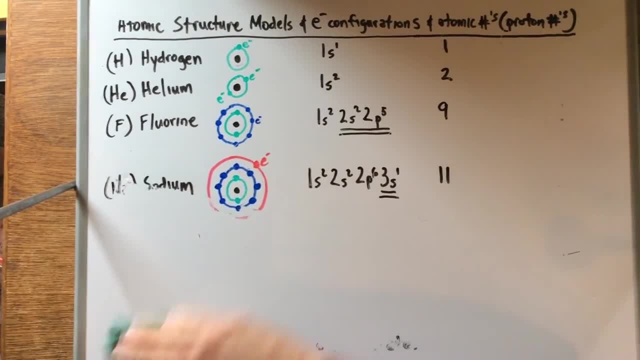 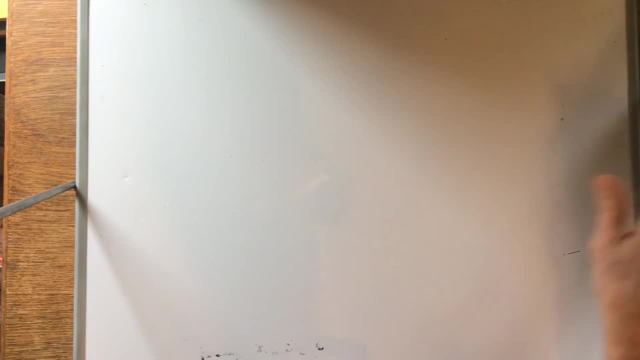 and show you a diagram, kind of a schematic, of what that's really about, how that works, because we're going to look at these. Okay, so these would be the electron energy states. All right, so we would start. if we're looking at energy increasing, going from bottom to 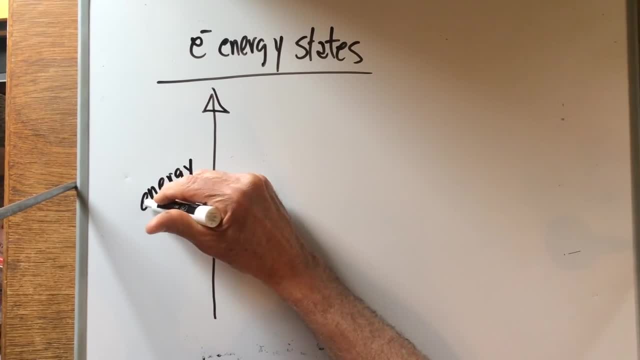 top. all right, then we're down here. we're looking at. the first one we have here was, of course, the 1s- all right, and then we moved up to 2s and then 2p- Again- the energy levels are increasing- and then we move up to 3s and 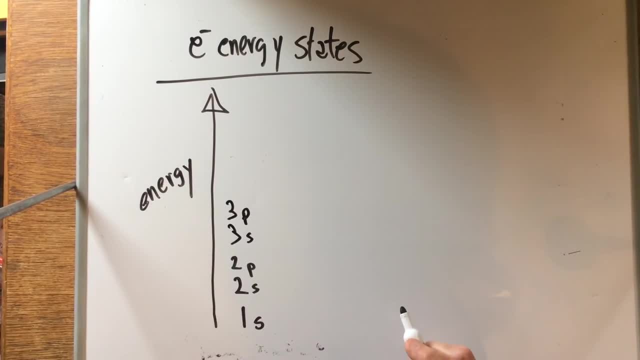 3p and there goes the timer. Now that also 3 has a d level to it also, but the d level is less energy than the 4s, So the 4s would go next. In other words, when you're doing electron. 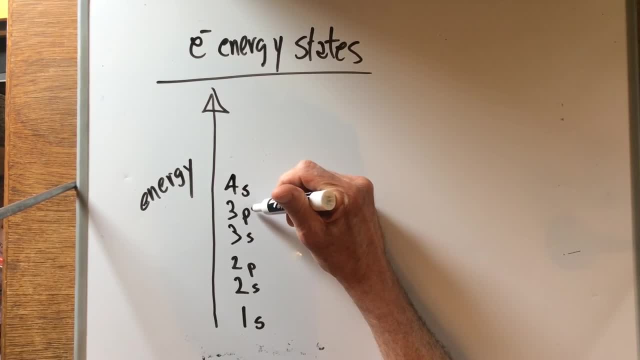 configurations. you wouldn't. after you fill up the p6, you wouldn't go directly to the 3d energy shovel. You'd have to go to 4s because it has less energy level than the 3d. So you'd. 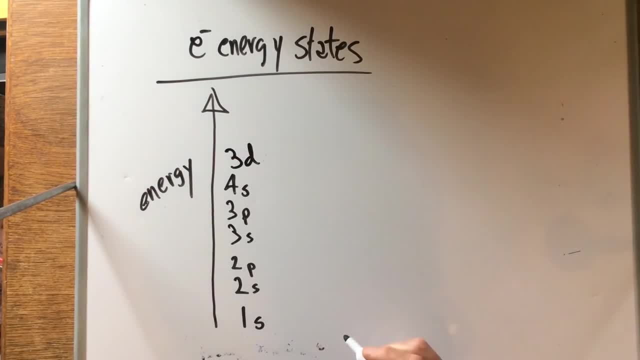 go 4s and then you would move up to the 3d and then keep going 4p, up to the 4d and then 4d, like that and on. okay, so this is the only little kind of hiccup right here is. 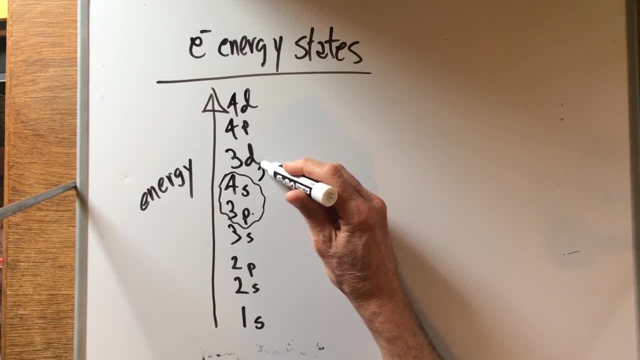 where you go from 3p to a 4s and then to the next available 3d. but it's not critical. but that's just when you see these electron states, you'll wonder why. what happened? what happened to 3d? while we're going, 4s begin. it's all about.